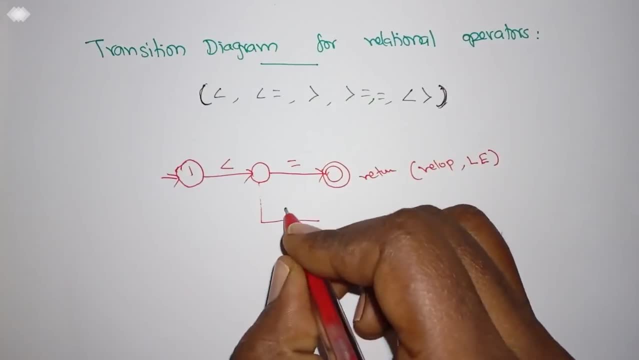 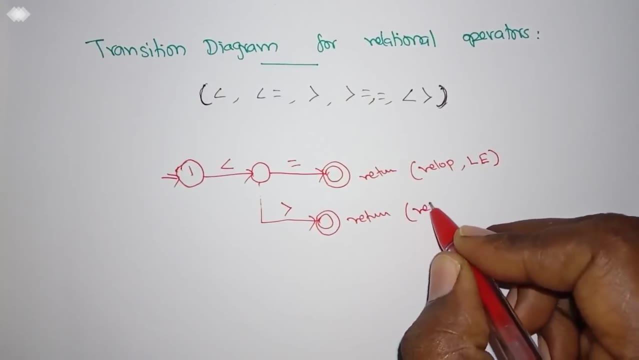 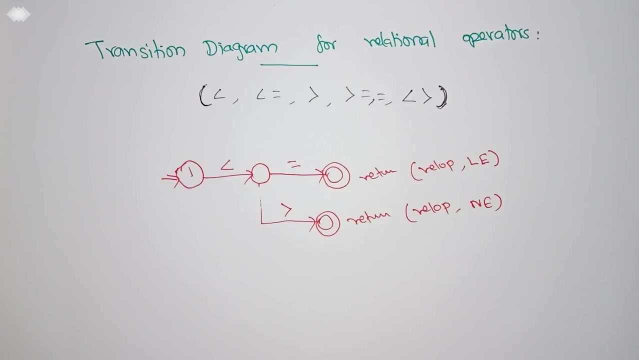 less than symbol followed by a greater than symbol. then also, we are going to return it as this final state and we are going to return it as relational operator. not equal to. It is a not equal to case, like it varies from programming language to programming language. that is what I 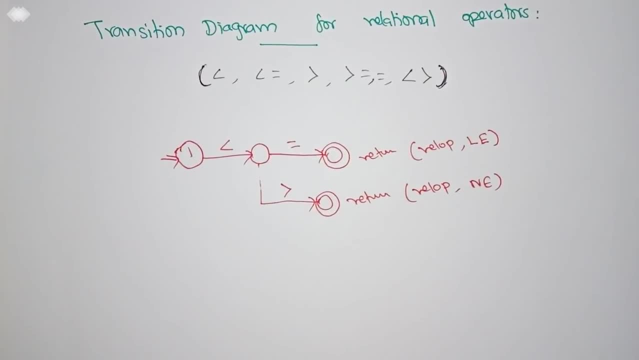 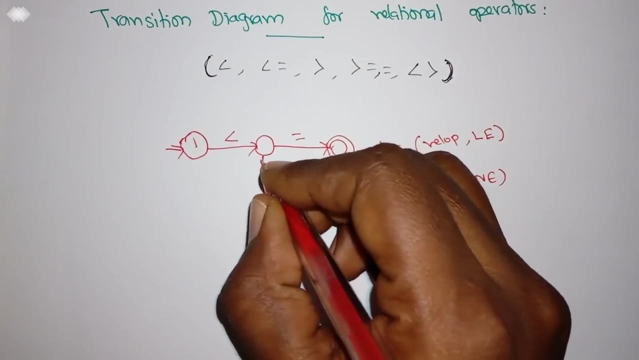 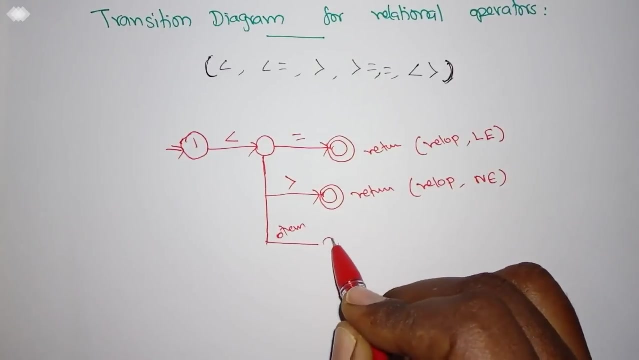 said right, It varies according to the programming language that I have taken. like this symbol actually denotes, it is a not equal to operator, or else if, instead of equal to or greater than, if there is some other symbols, Then you are going to make it like you are going to strictly say that it is a strictly less than symbol. 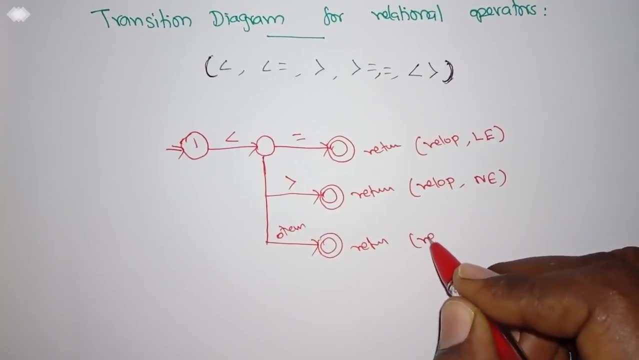 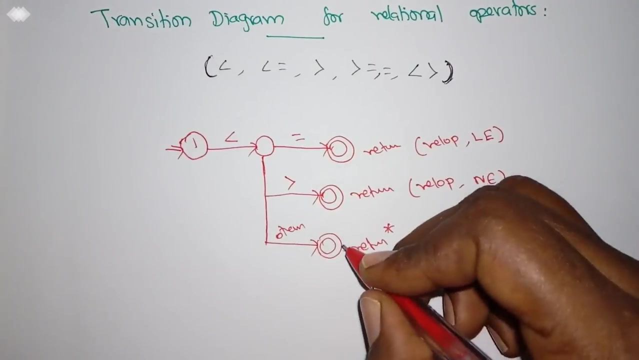 Okay, so you are going to return. it is a relational operator less than. but the problem here is we have read one more character of next lexeme to process this right, so that has to be returned back. So we use this asterisk symbol either towards here or towards here. that actually denotes we have to move a step back for the next processing. 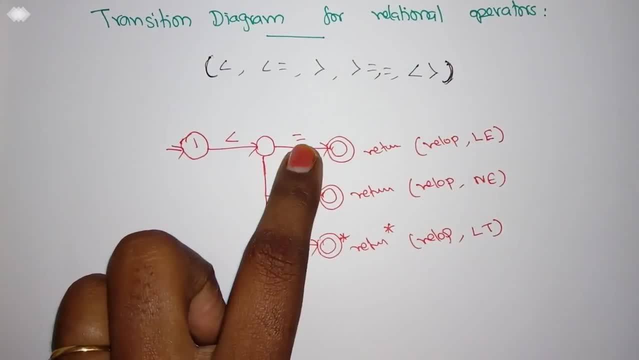 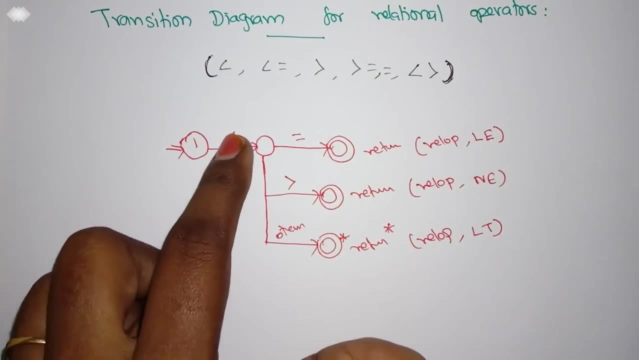 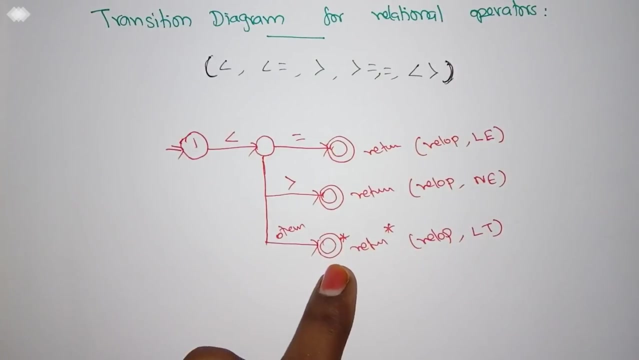 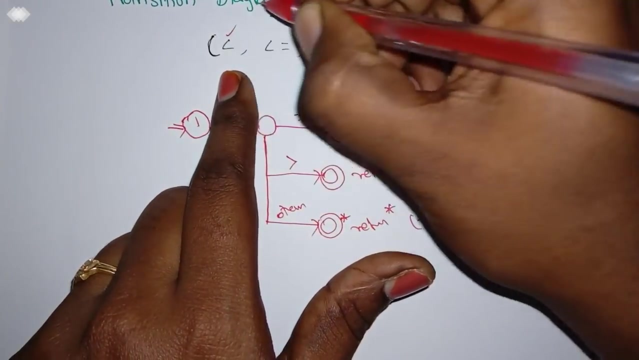 Okay, So here it is less than or equal to. both are involved in a lexeme. okay, the lexeme is less than equal to and the token is it is a relational operator, le, and here only the less than is a lexeme, and this is a part of next lexeme that you want to read. okay, in that case we have to move a step backwards for processing. okay, so this is one step. when it is less than or less than, or equal to or not equal to case, and similarly, when you have a greater than condition. 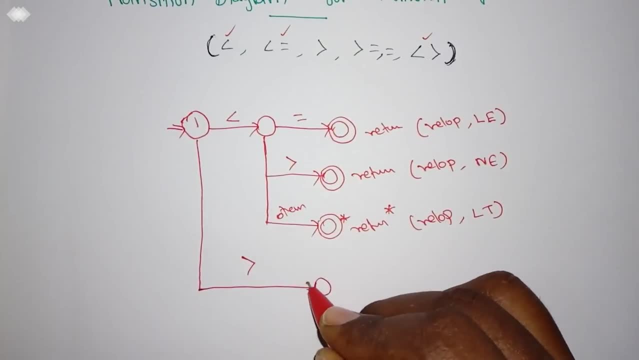 Okay, Greater than. you have two possibility. either it might be a greater than, or greater than or equal to condition, so you have to read the next element to recognize it. if the next element is equal to, what does that means it is a relational operator reload. and next one is: if it is greater than equal to, we are going to return it as greater than equal to criteria. okay, and one more possibility of greater than or equal to condition.